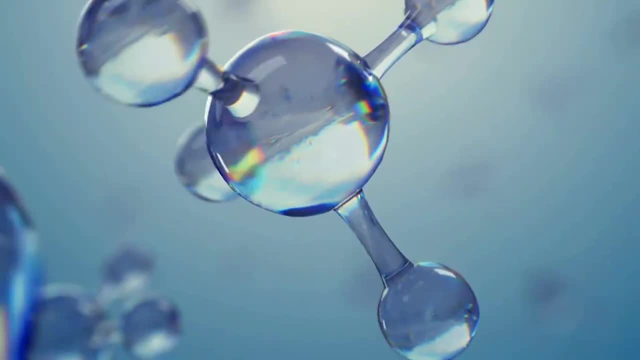 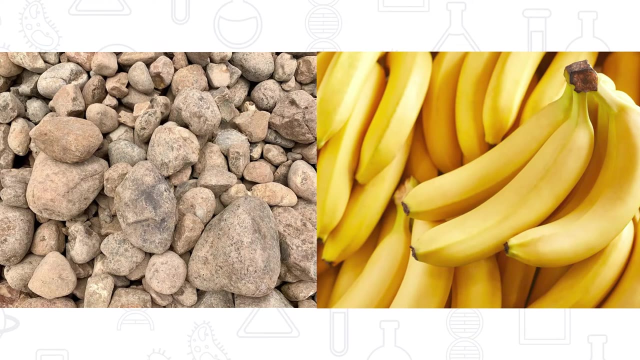 Depending on the way that atoms interact with each other and are bonded together, they can create anything. Let's compare a rock versus a banana. They're two completely different things with different shapes, colors and textures, But they're both made up of atoms. 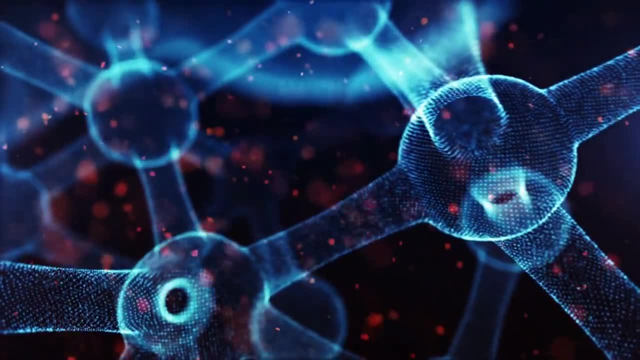 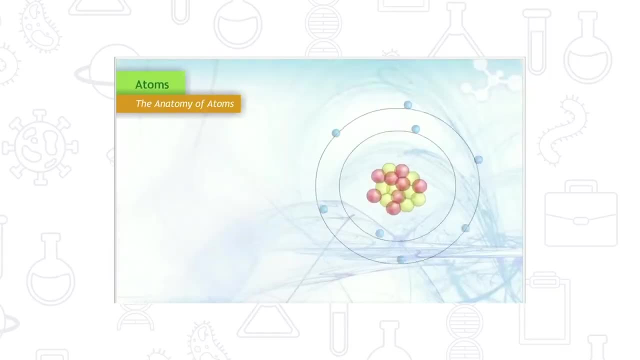 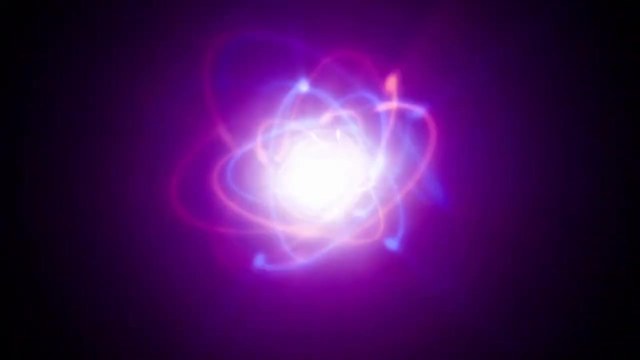 Starting with just a very small particle. the way atoms interact with each other can dictate what the object could be. How cool is that? Looking inside an atom, it has a central core called a nucleus. A nucleus is made up of protons and neutrons. Electrons are charged up with a ton. 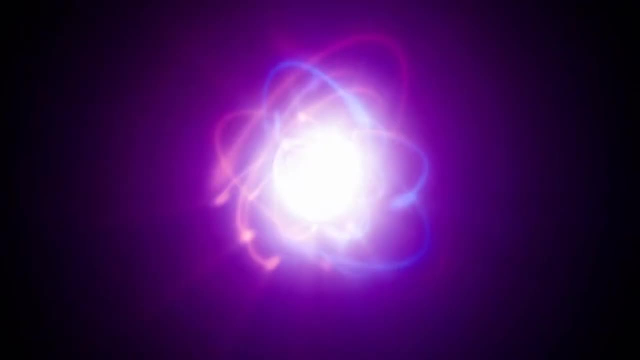 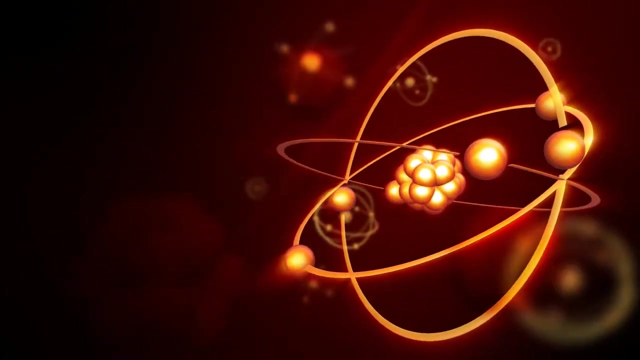 of energy and these negatively charged particles spin around the outside of the nucleus. The nucleus is like the Sun. The electrons are planets orbiting the Sun. The cosmic particles follow theолн the Sun. What makes atoms different from each other? What really makes atoms? 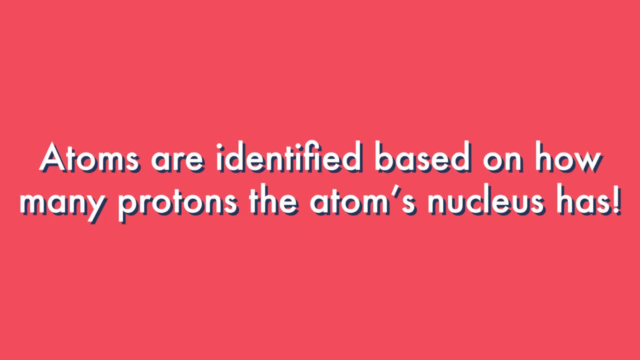 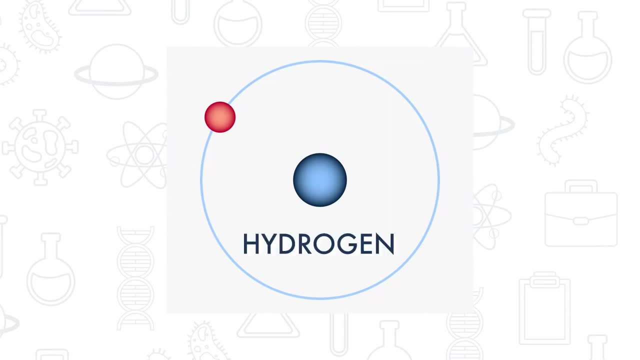 different from each other is how many protons each atom's nucleus contains. For example, when an atom has one proton in its nucleus, it becomes a hydrogen atom. When an atom has two protons in its nucleus, it becomes a helium atom. When 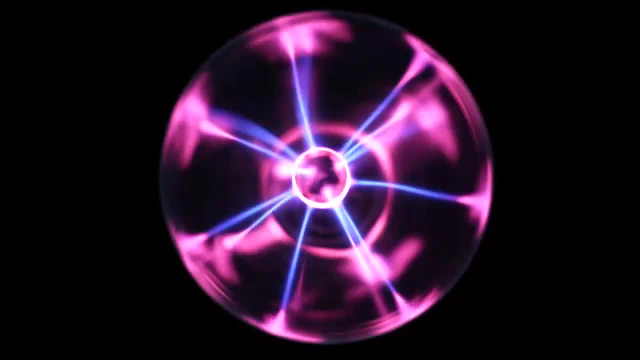 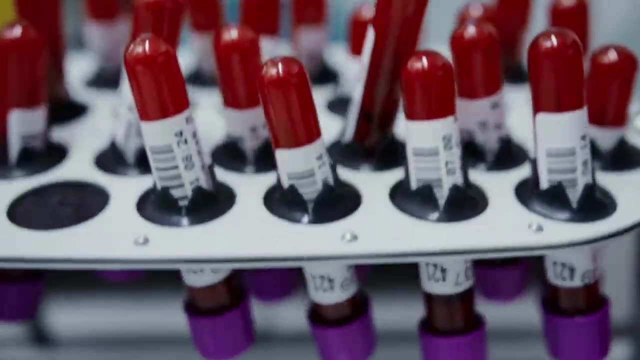 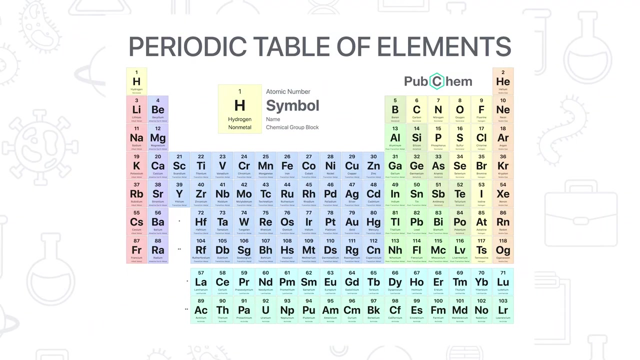 you know how many protons are in an atom, it becomes a specific element like hydrogen and helium. These elements are the simplest forms of matter and help dictate the physical properties of their substance. Have you ever heard of the periodic table before? This table lists all of the chemical elements in the 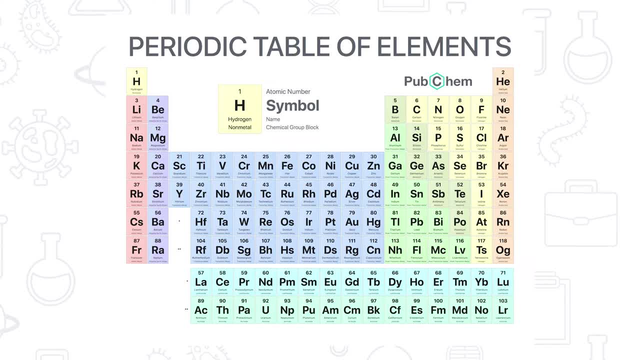 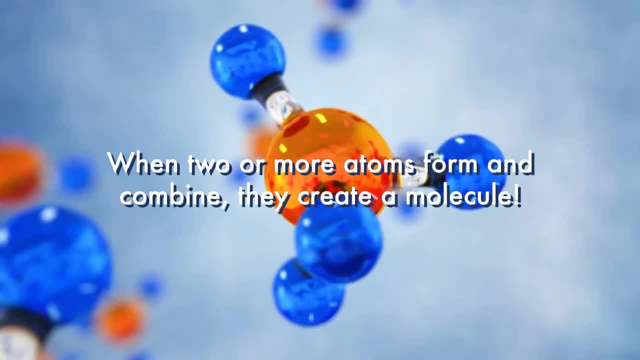 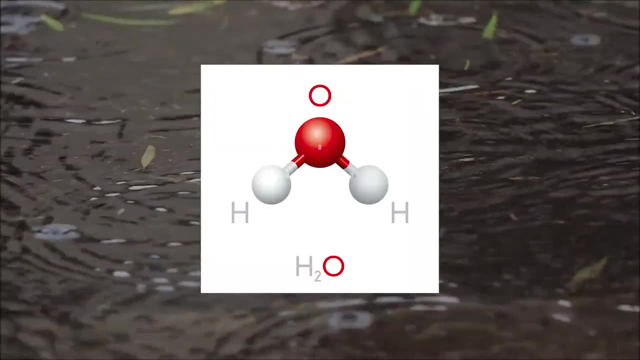 world and in the order of how many protons and atoms each nucleus has. When two or more atoms form and combine, they create a molecule. The most common molecule that people refer to is H2O or H2O Water. The H is hydrogen and the O is oxygen. That means water molecules have 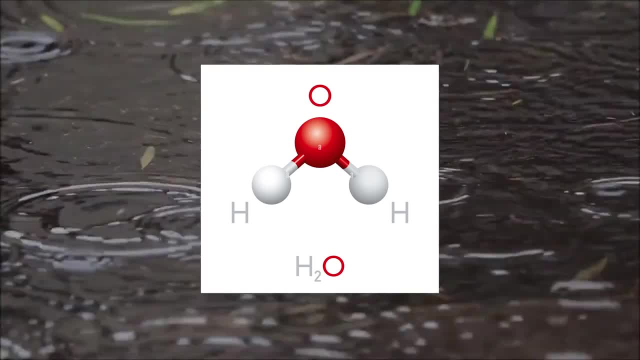 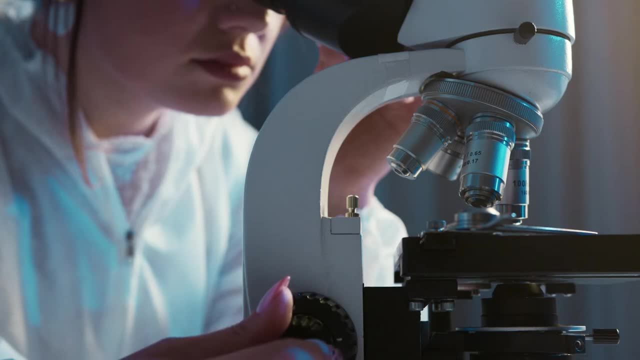 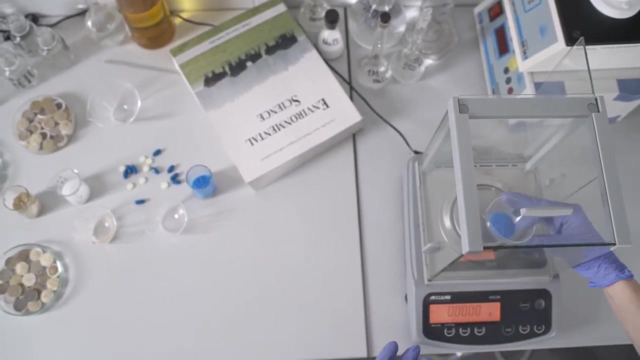 two hydrogen atoms and one oxygen molecule. There are so many different kinds of chemistry, but chemists study atoms and molecules to understand everything in the world and how it works. Chemistry is often referred to as the central science because it joins together physics, math, biology, medicine. 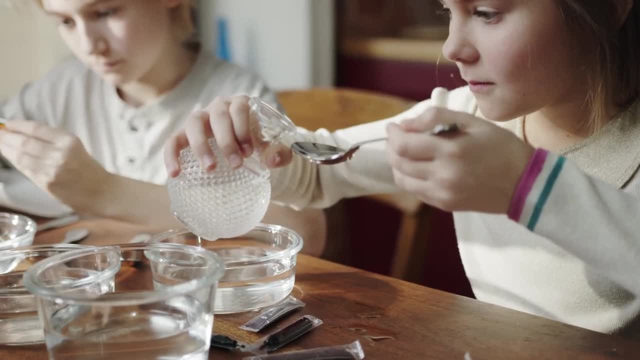 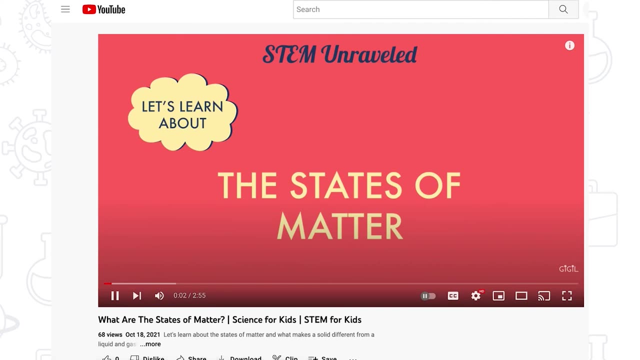 and so much more. We hope you enjoyed learning all of this. See you next time. Bye about the basics of chemistry. There's so much more to learn about out there If you want to learn about how atoms make up the states of matter.